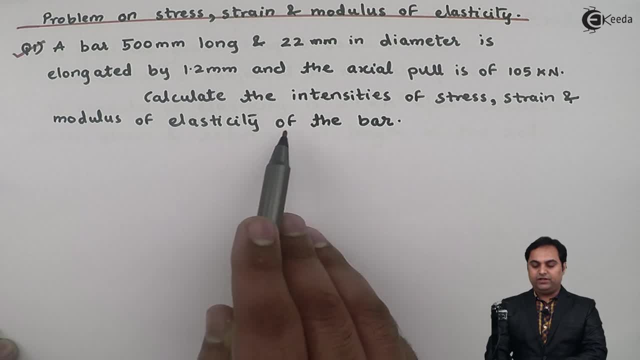 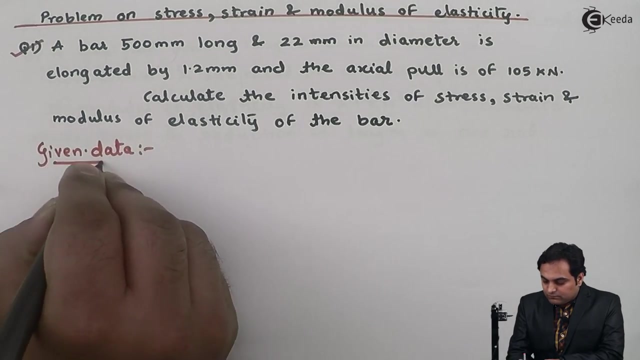 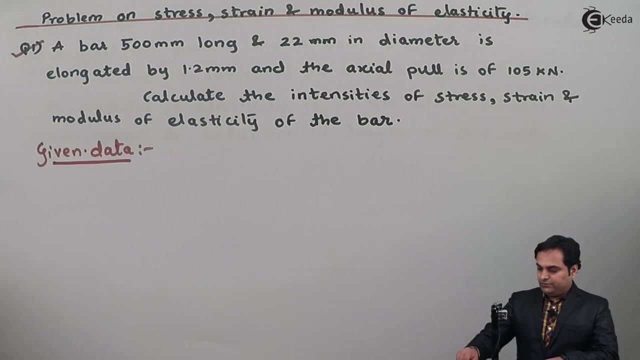 the intensities of stress, strain and modulus of elasticity of the bar. This is the question in front of us. First of all, whatever is there in the question, we will write that in the form of data. Let us get started Now. it is given a bar is 500 mm long and 22 mm in diameter. 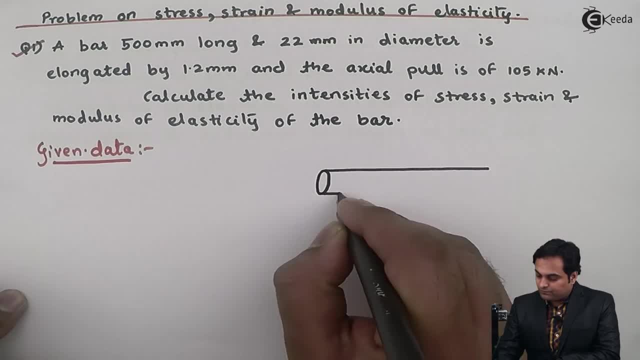 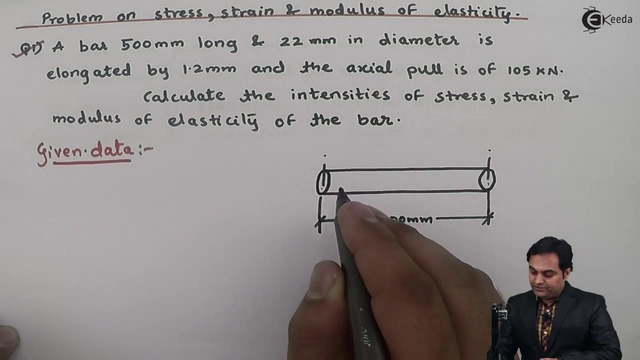 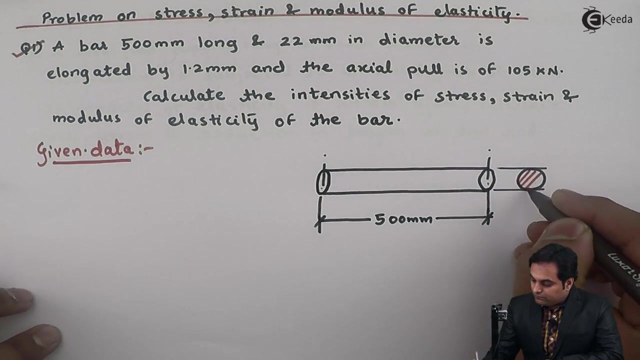 I will draw the diagram for the same. Here I have drawn a bar or a rod whose length is 500 mm and diameter is: if I look at this cross section here, this diameter is 22 mm. So the bar having length and diameters is elongated by 1.2 mm. This elongation means: 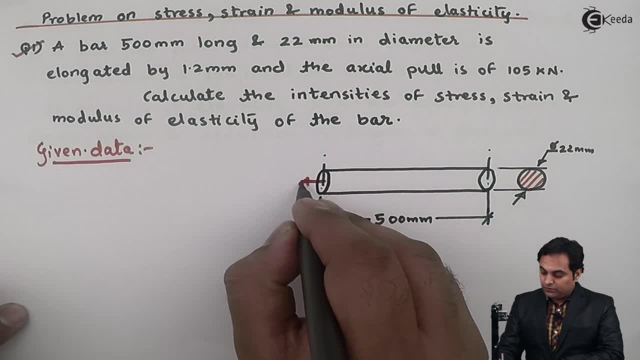 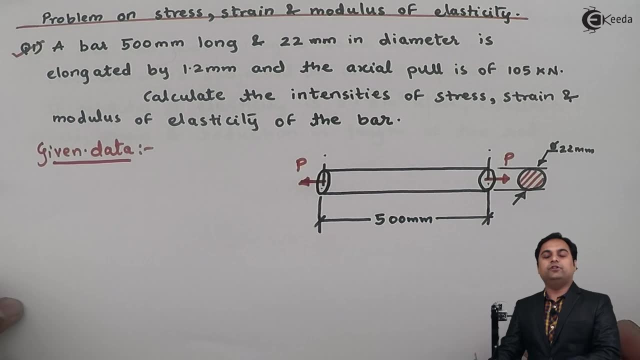 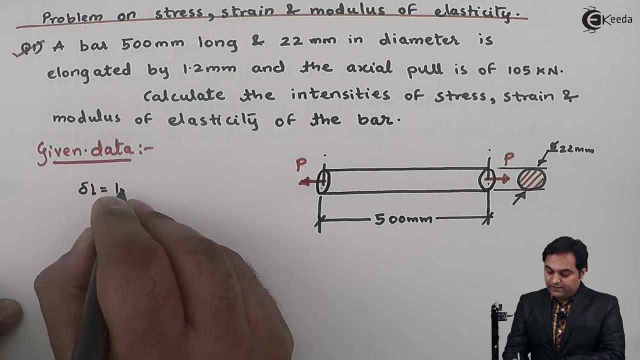 that here over this bar there would be a pull type of load. that is why there is elongation. So here P indicates the pull type of load on the bar and elongation is given as 1.2 mm. Elongation is denoted by delta L, that is 1.2 mm, and the axial pull is of 105 kN Value. 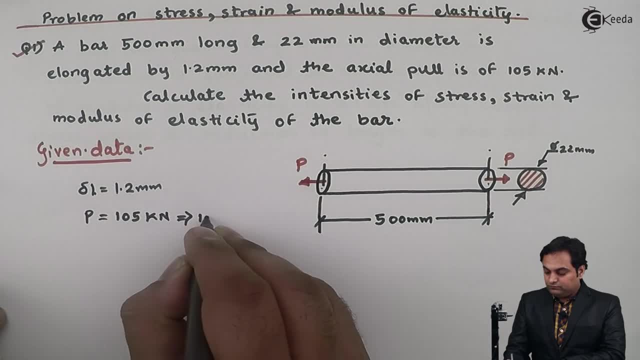 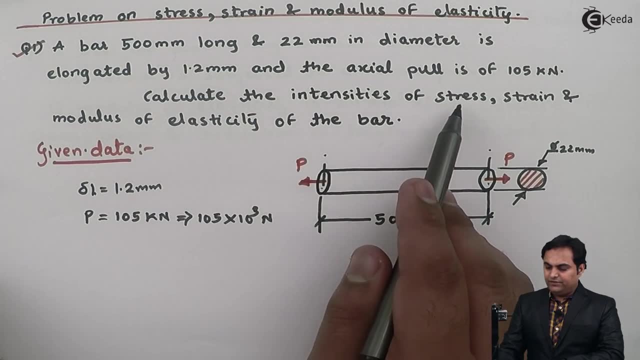 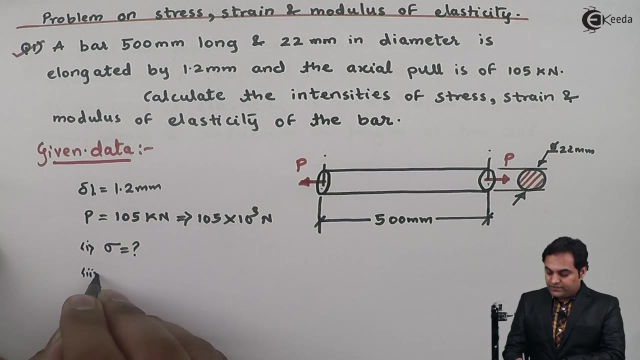 of P is given 105 into 10, raise to 3. N. Calculate the intensities of stress. The first question is to calculate the value of stress, And third, we have to calculate the modulus of elasticity of the bar. So this is the question in front of us. Whatever was given here, we had written that in the 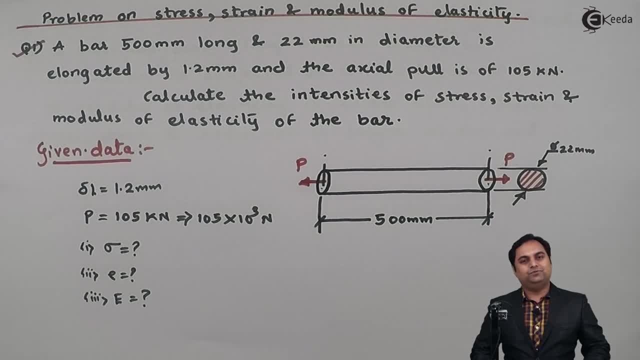 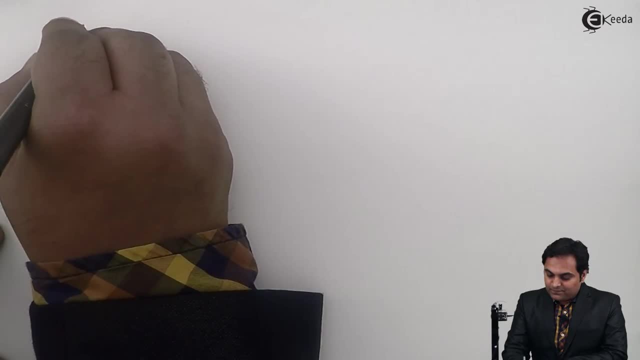 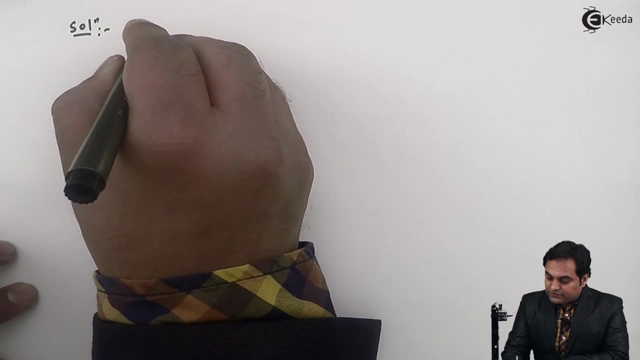 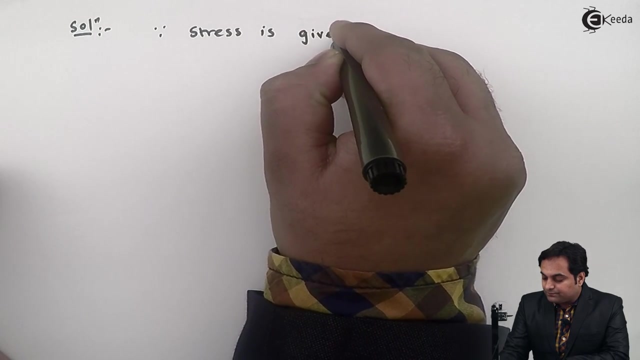 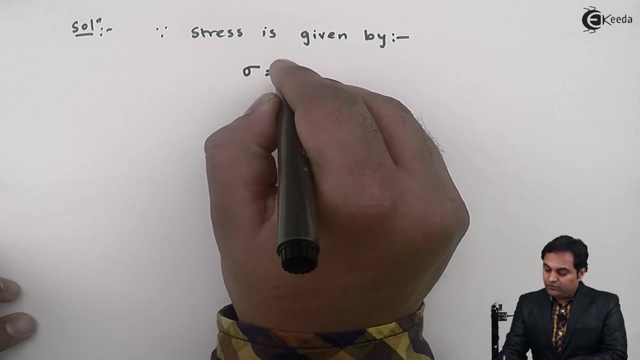 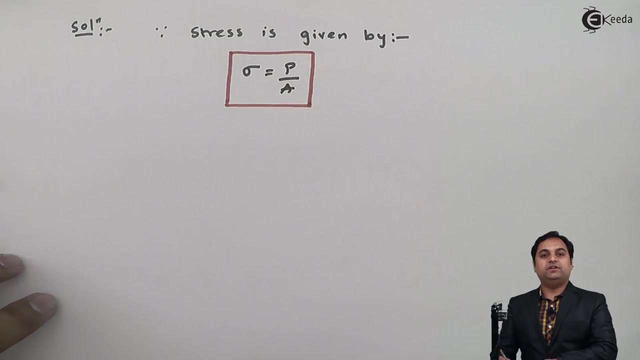 form of data. Now let us try to get the solution to this problem Now in the solution, as the first question is stress. So I'll say that, since stress is given by the formula is sigma is equal to P upon a. So this is the relation Now when we look into 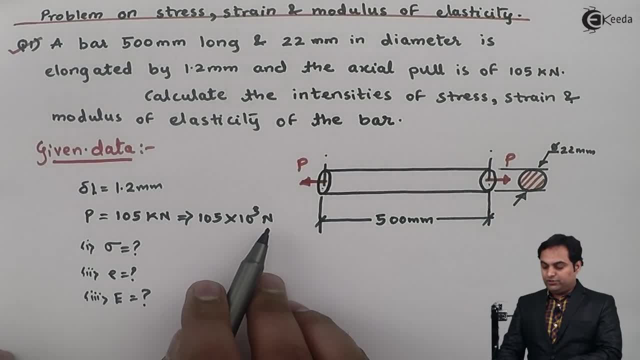 this question. P is equal to 0.42 times 0.42 times來到 the 0 Yuan scale, 1 full放解. P is given as 105 into 10. raise to 3 Newton and area. we can get it from the diameter diameter. 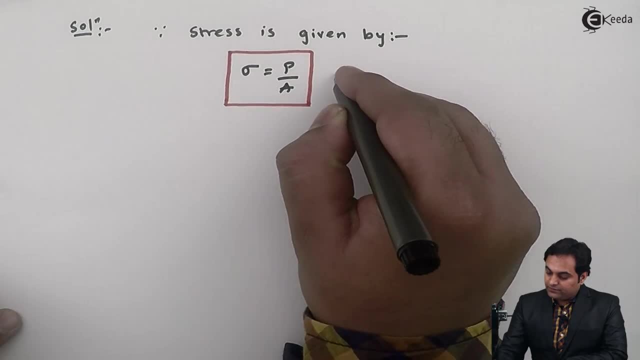 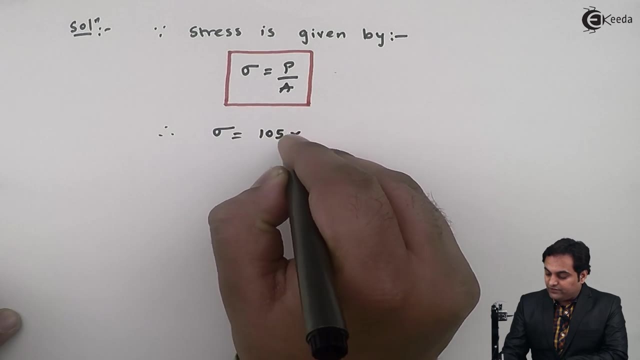 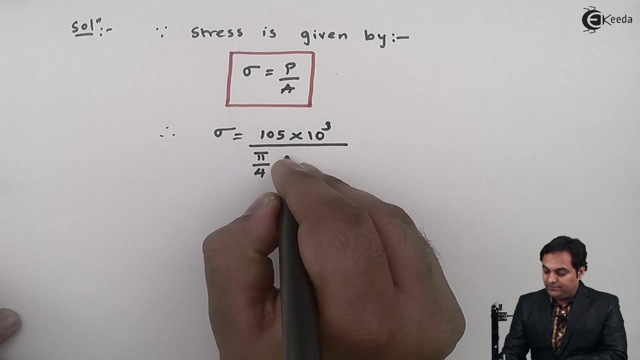 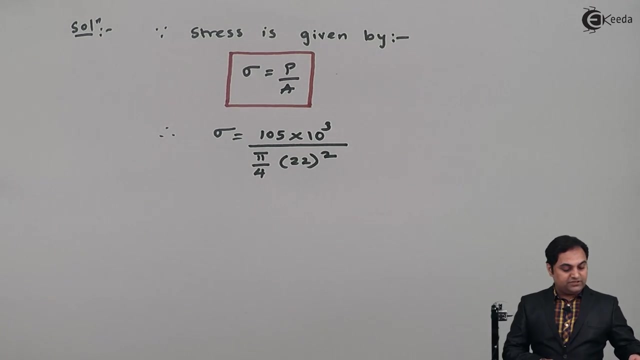 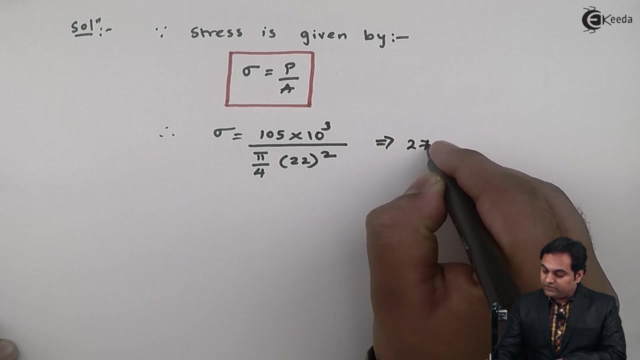 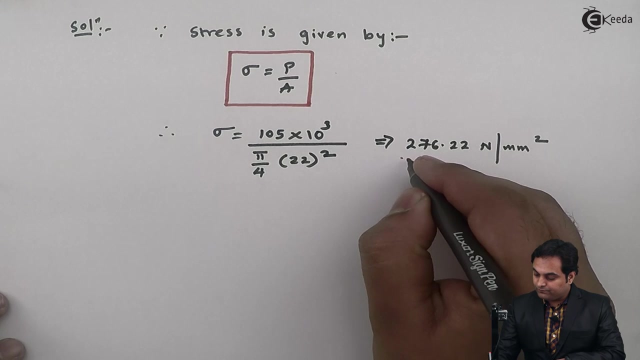 is 22 mm. so here I'll write down this: stress Sigma will be equal to P, is 105 into 10. raise to 3 Newton area, it is pi by 4 into diameter, which is 22 square, and from this I'll get my first answer of stress, and that answer is 276.22 Newton per mm square. this is the 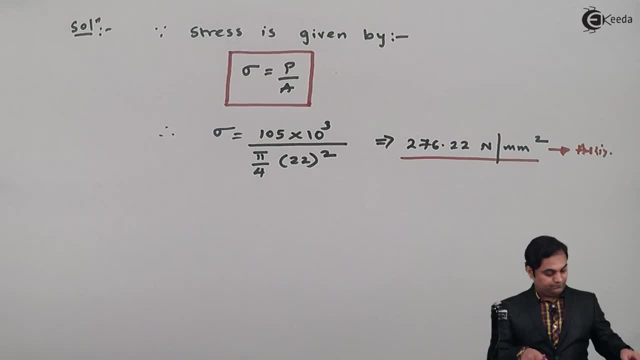 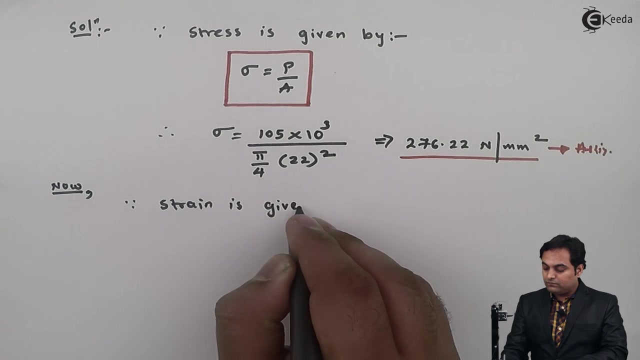 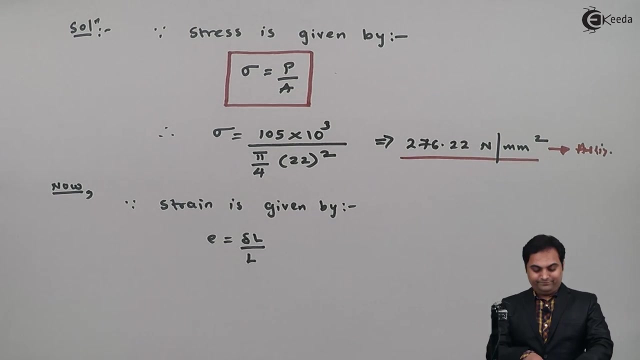 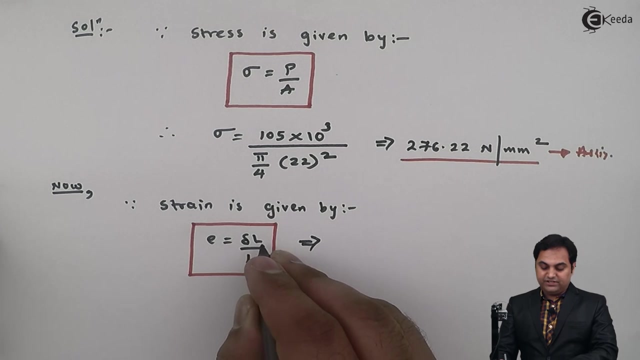 first answer. Next they are saying us to calculate strain. so after stress, I'll write down now, since strain is given by the formula is: strain is equal to change in length upon original length. so here I'll put the values. change in length is given in the problem. it is 1.2. that is the 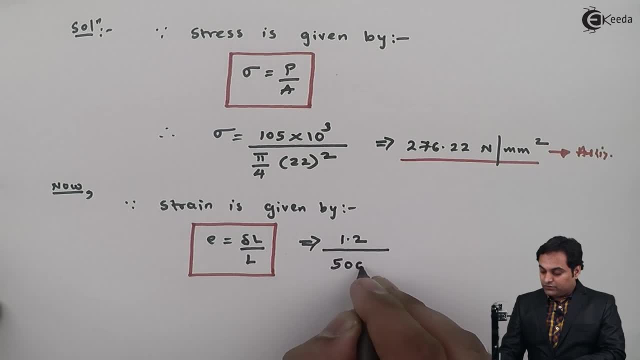 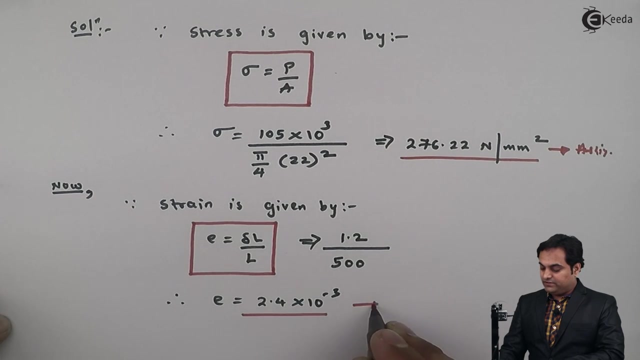 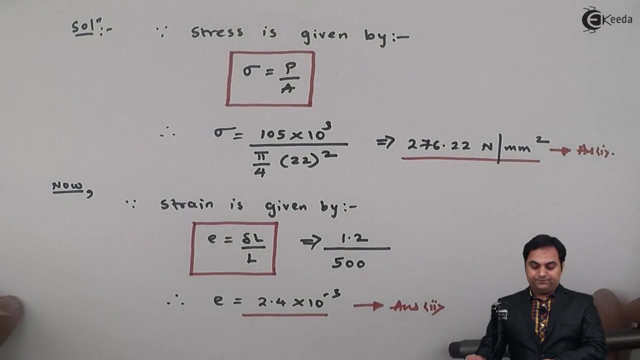 deflection and length is 500. so from this I will get strain. it comes out to be 2.4 into 10, raise to minus 3 and strain won't have any units. It is A dimensionless quantity. Next, after getting strain, 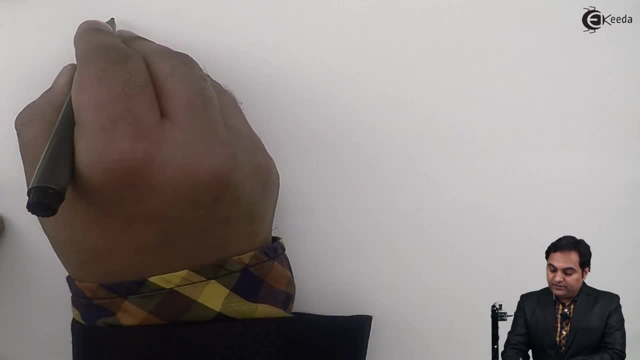 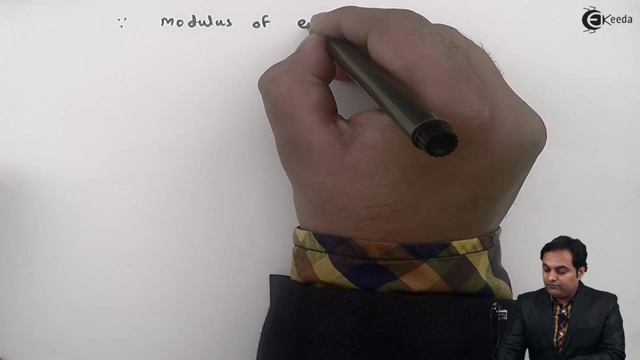 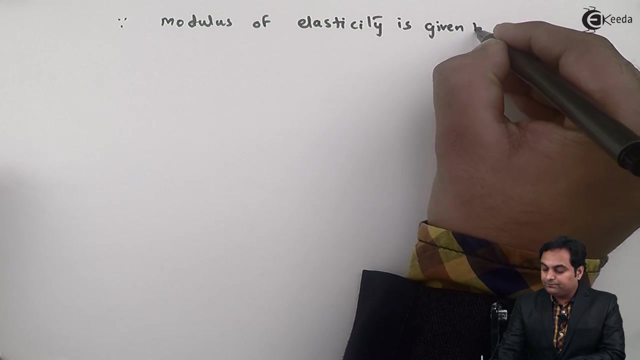 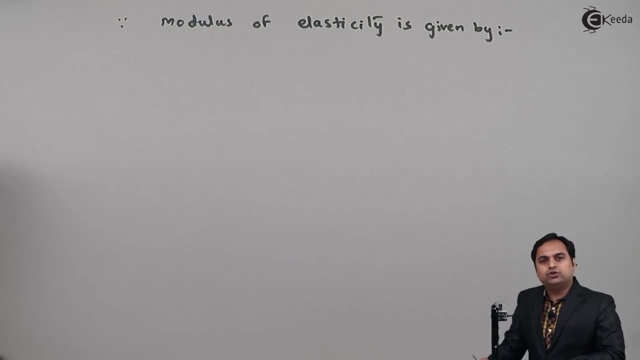 The third part is modulus of elasticity. so I can say that since Modulus Of elasticity Is given by Modulus of elasticity, We can Get it from Hooke's law. in Hooke's law it was modulus of elasticity was equal to stress. 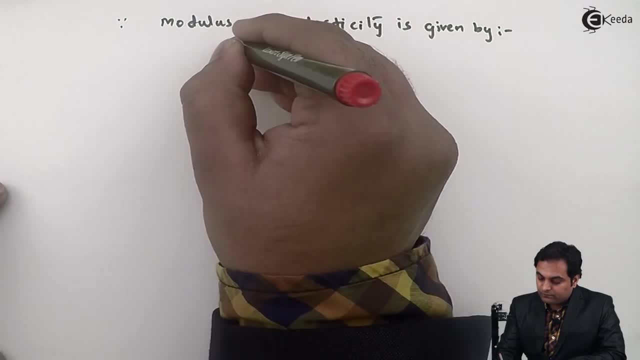 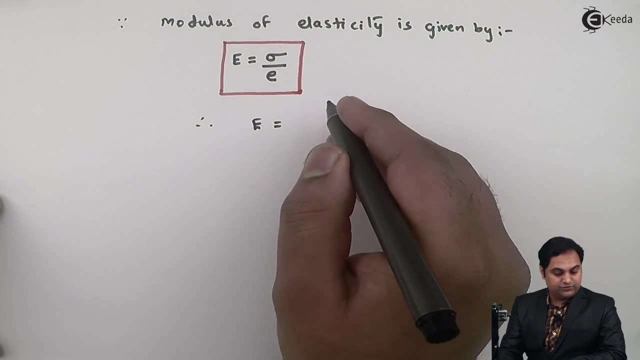 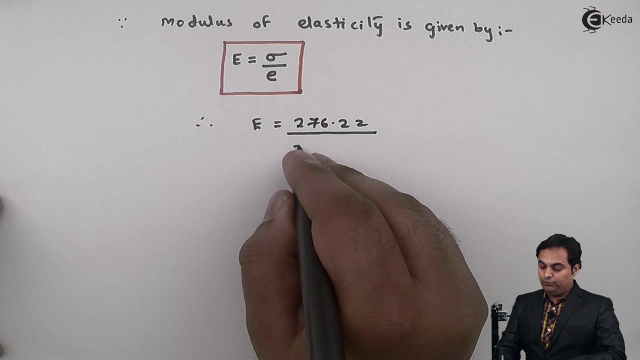 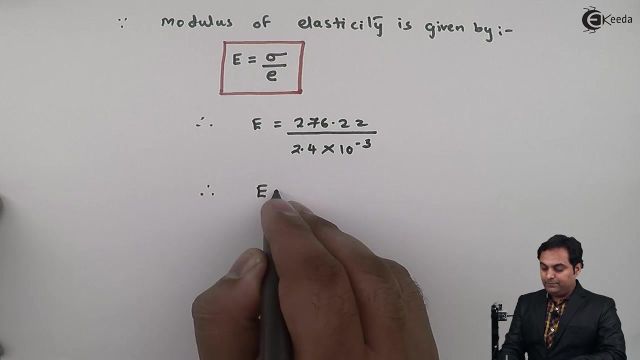 upon strain. So here I'll put the values. therefore, Young's modulus is equal to stress, is 276.22. our answer number 1: strain 2.4 into 10, raise to minus 3.2.. So From this I will get capital E, Young's modulus. my answer is: 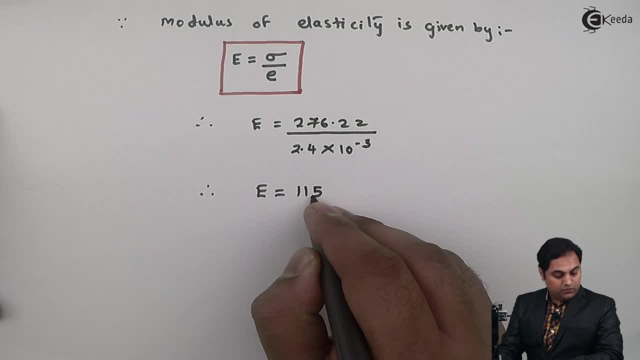 It comes out to be 1, 1, 5, 0, 9, 1. Point 6: 7. Newton per mm square. So this is the answer of Young's modulus, or you can say modulus of elasticity. So 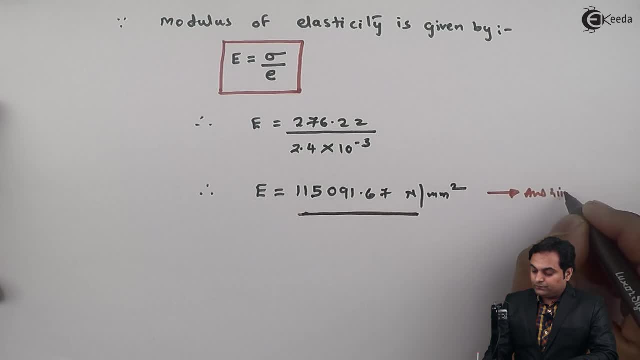 If I write the answers at the end Here we have Got stress as Two seventy six point two two Newton per mm Square. Answer number 1.. Strain 2.4 into 10, raise to Minus 3.. 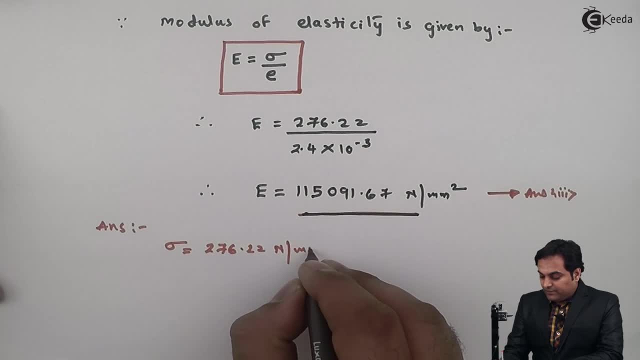 Second answer: And Young's modulus And it is equal to the new. The amount of stress That we got Here we have 2. 6. N N Newton per mm. Square. Answer number 1.. 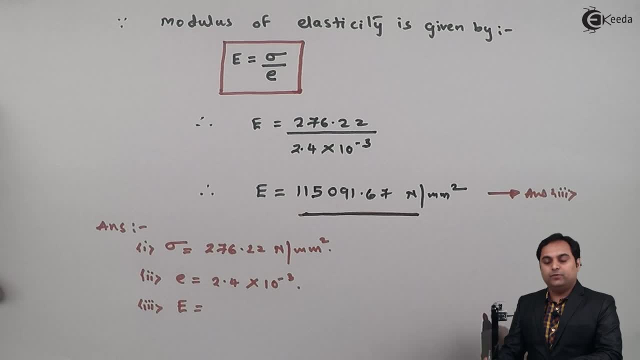 Strain 2.4 into 10 raise to Minus 3.. Second answer: And Young's modulus. This value 1, 1, 5, 0, 9, 1 point 6, 7 Newton per mm. square. so here we have completed the. 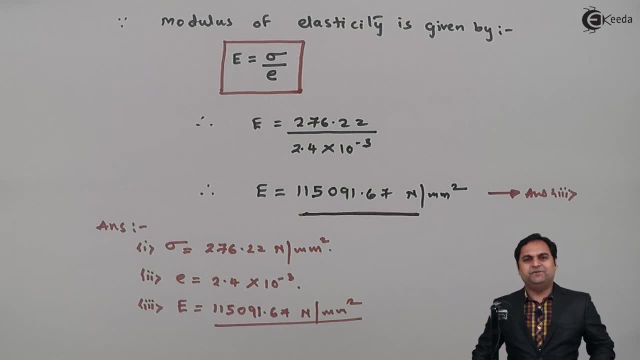 problem, that is, we have calculated whatever values. that was unknown.